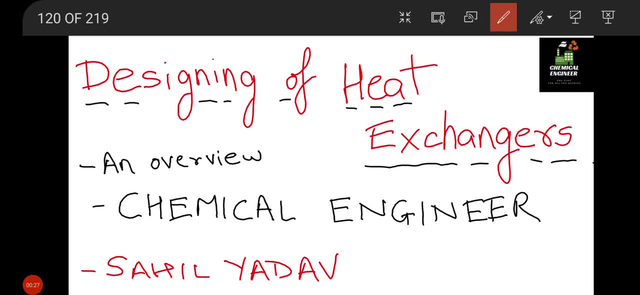 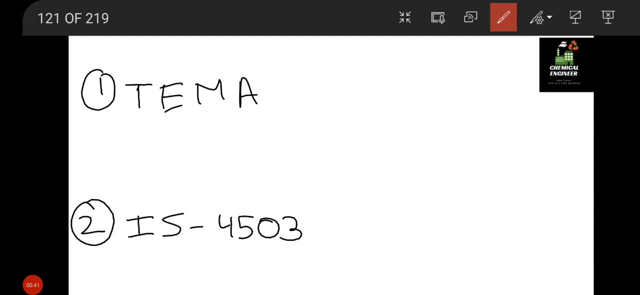 here we will be covering shell and tube type heat exchanger. so if you haven't subscribed to us till now, please subscribe us and let's start the video. so in order to design heat exchanger, we have two standards. first is TEMA- you can call it as TEMA. second is is 4503, so I am talking only about 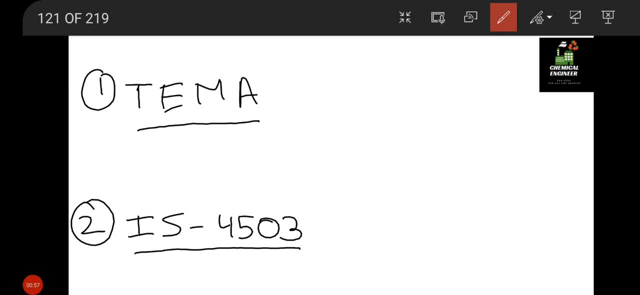 Indian standards or which is followed in India. so TEMA stands for tubular exchanger, tubular exchanger, manufacturing association. so manufacturer, manufacturer association. okay, so this is in USA. okay, so this is in USA. so all the heat exchanger, or all the things that we are going to define for heat exchanger, is based on this TEMA. that is TEMA tubular. 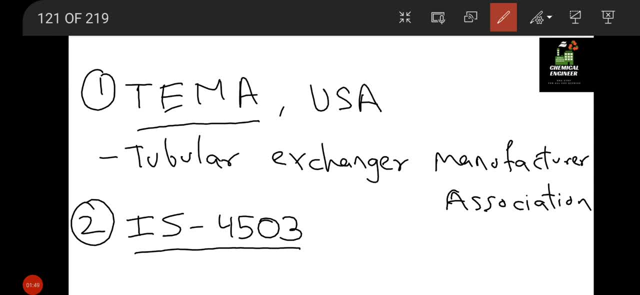 exchanger manufacturing manufacturers association and is 4505 stands for Indian standard standards 4503. so Indian standards 4503 is almost equal to TEMA of USA. so what? all things are required to be designed for heat exchanger. so let us see their names, and from: 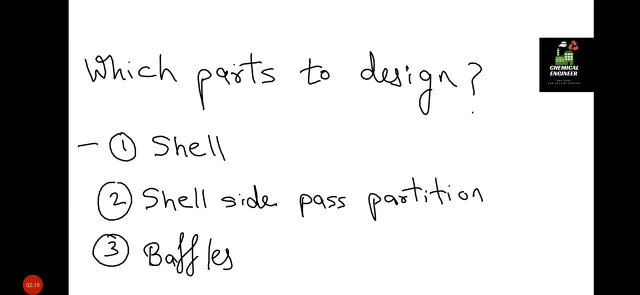 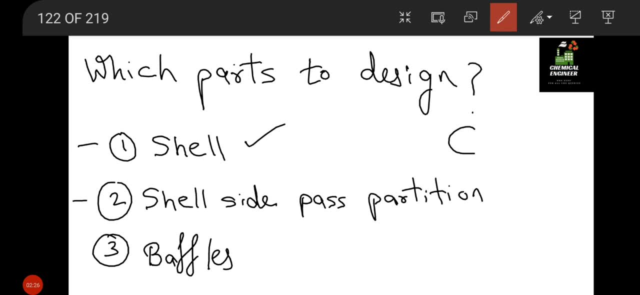 the next video we will cover all of them. so which part to be designed? so we start from shell. so basic outlet of the heat exchanger is shell. okay, so we will see how the diameter is designed for shell. what is the thickness required for the material of the shell? this thickness and 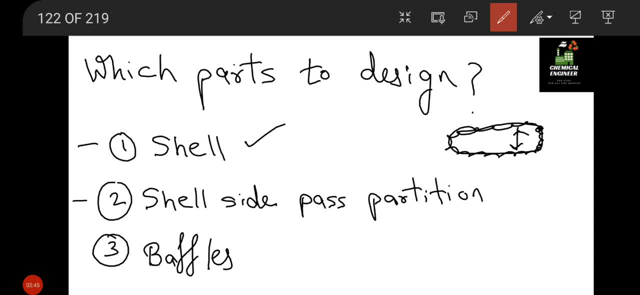 then we will see about the clearance that is required for the expansion or contraction, and so we will also see how we can adjust tubes inside that shell. so based on that, we will see from the next video. first video will be of shell. we will design shell of heat exchanger. next we have shell side pass. 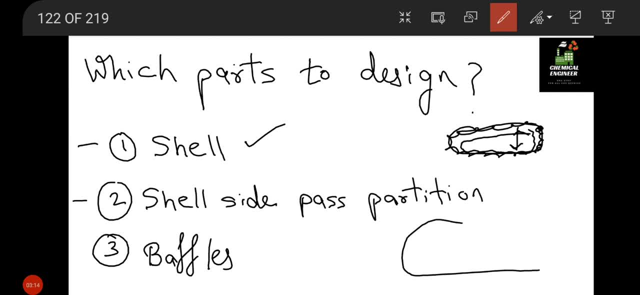 partition plate. okay, so suppose this is a shell here, suppose this is the shell inlet. so we will have various passes like: suppose this is coming in and this is going out like this: so this is single pass. now if we want to increase the passes or to enhance the heat transfer, we can make it multiple pass, like this: 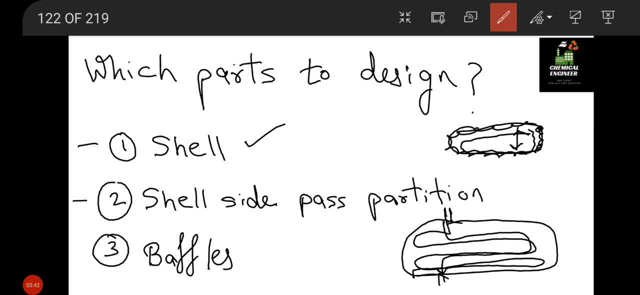 okay, and then coming out from there, only so multiple pass and single pass we will cover in the next video. so this is second shell side. pass partition. third is is basis, believe me, basic done. we'll cover it just one more time, okay. so next in the third video of 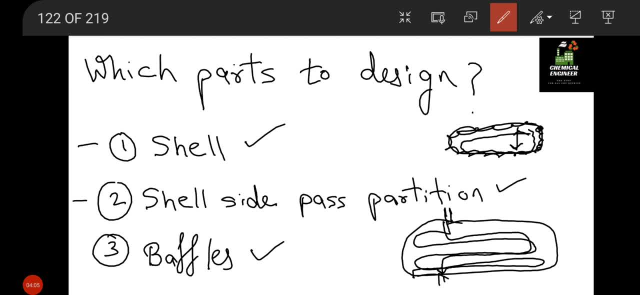 these courses. we will cover baffles. third, of course, is efficiencies of method for heat exchanger and thr vote that baffles has baffles case. we will cover first one in today's fourth of course, acre power baffles and then the second video of third component baffles. so there is is. 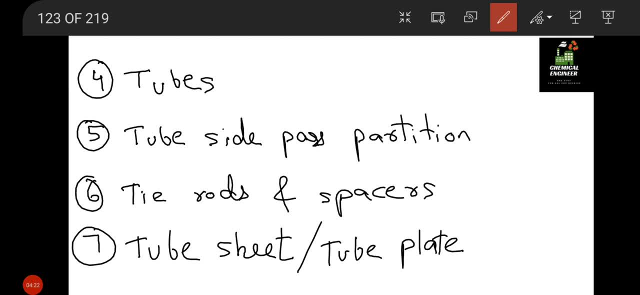 baffles U sports quel Roland, baffles savers32 and baffles schumipa. 262 is an example of different heat exchanger. we will cover about tubes, so we will see how we can design a tubes or in tubes. we will design thickness and diameter, so we will design thickness and. 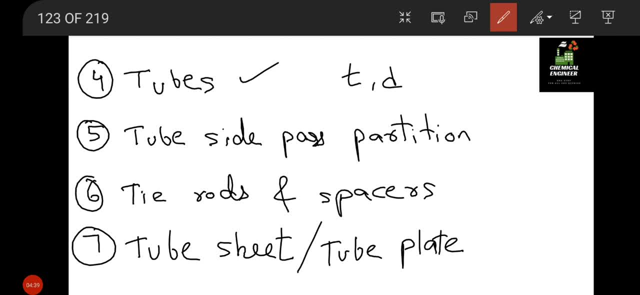 diameter for tubes. similarly, tube set pass partition. so we may have tube single tube like this. we may have a curved tube like this, YouTube we can call it. or we can have different arrangement of tubes inside a shell. we will see about it in the third video. so all this thing will be covered.